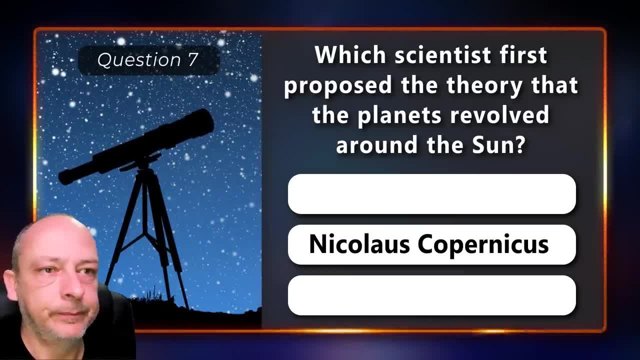 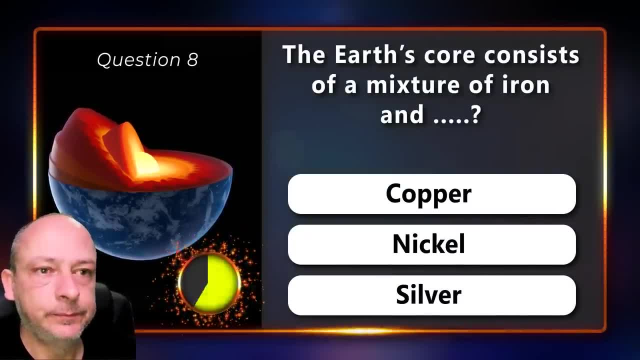 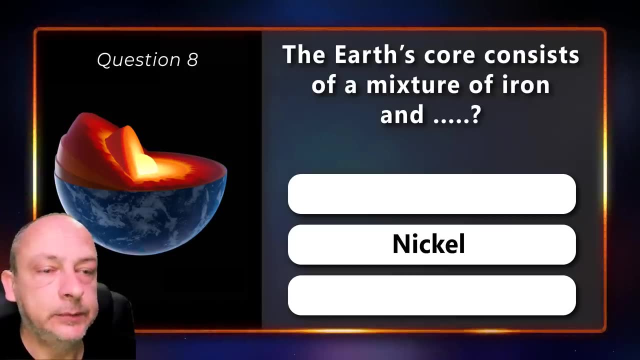 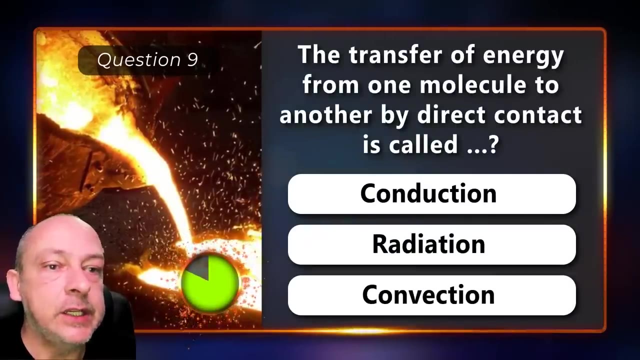 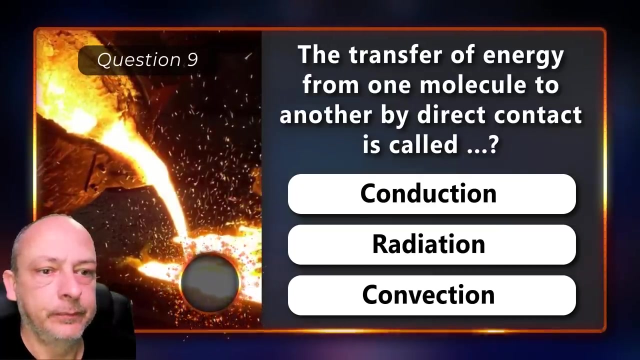 Nikolaus Copernicus, The Earth's core consists of a mixture of iron and copper, nickel or silver. The answer is nickel. The transfer of energy from one molecule to another by direct contact is called conduction, radiation or convection. It is conduction. 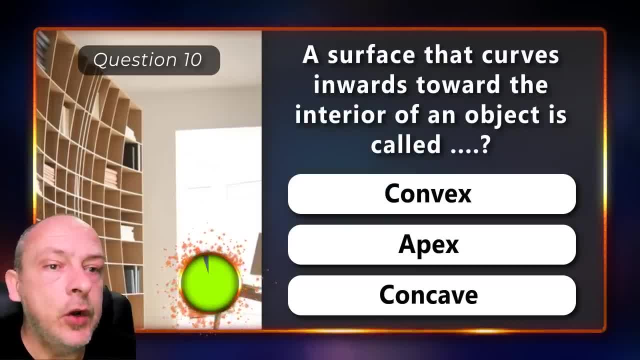 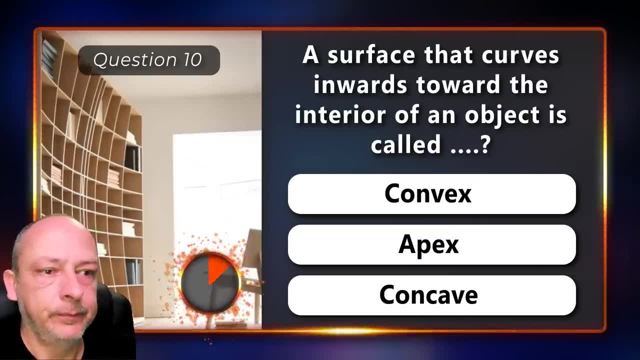 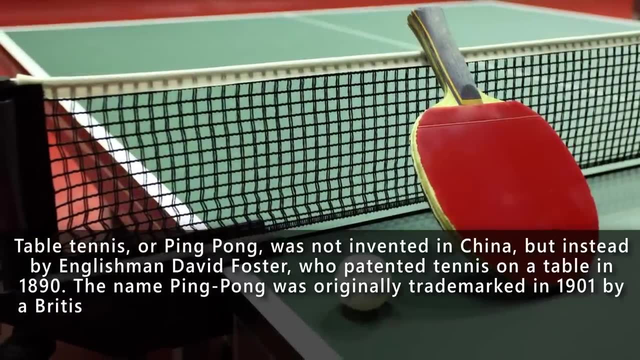 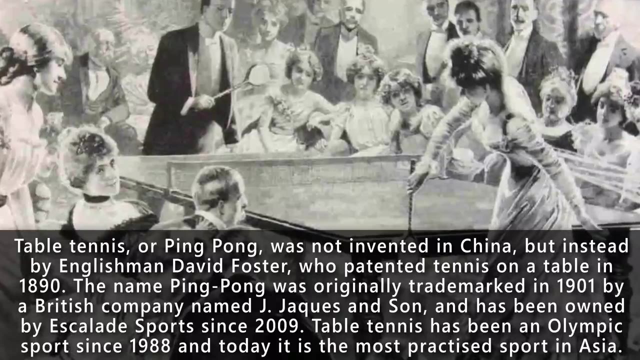 A surface that curves inwards towards the interior of an object is called convex, apex or concave. It is concave, Not a science fact. but did you know that table tennis or ping pong was not invented in China, but instead by Englishman David Foster, who patented tennis on a table in 1890. 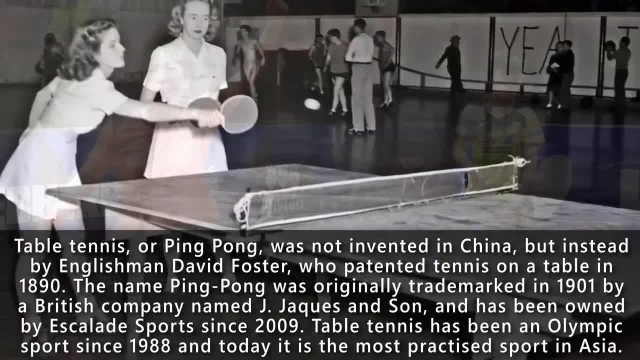 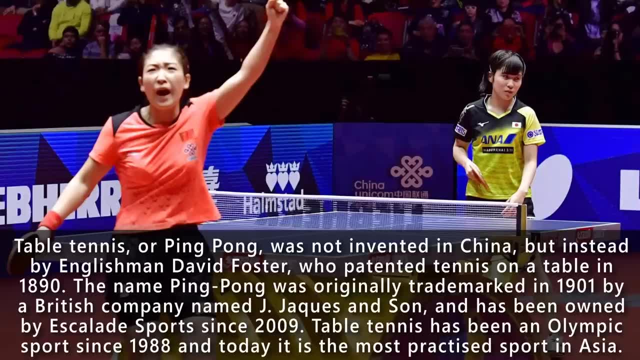 The name ping pong was originally trademarked in 1901 by a British company named J Jacques & Son and has been owned by Escalade Sports since 2009.. Table tennis has been an Olympic sport since 1988, and today it is the most practiced sport in Asia. 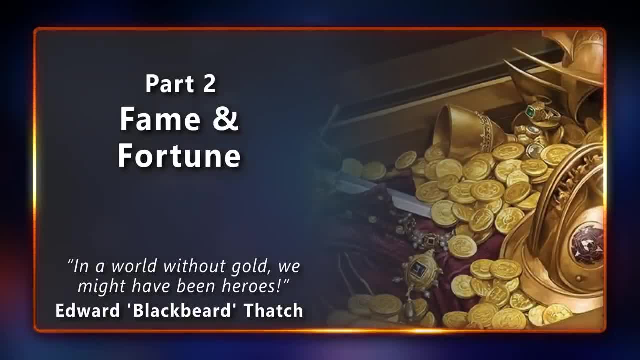 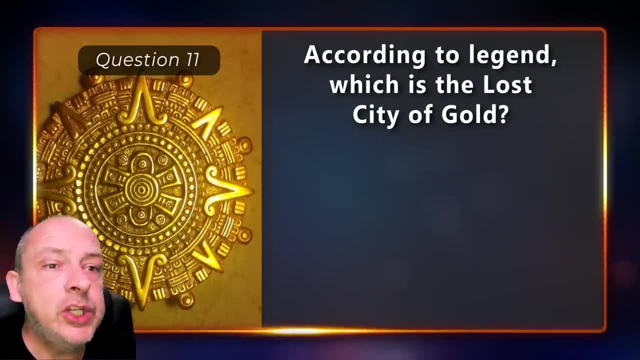 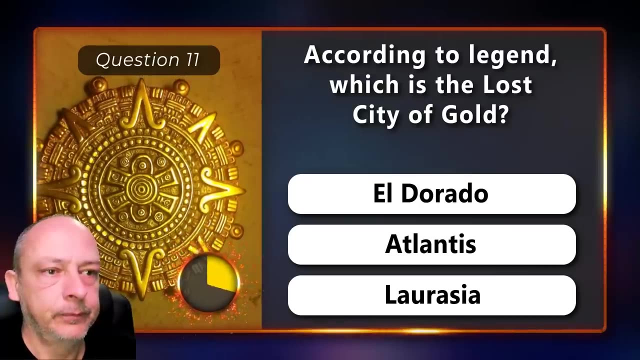 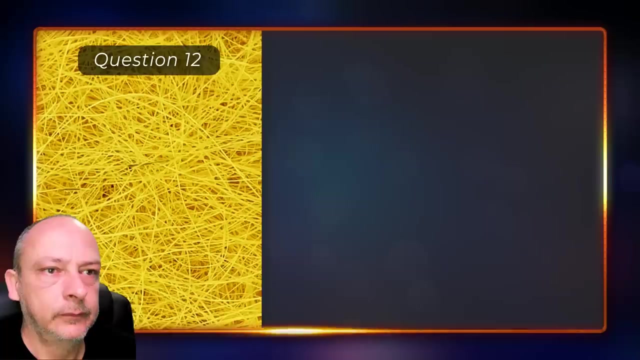 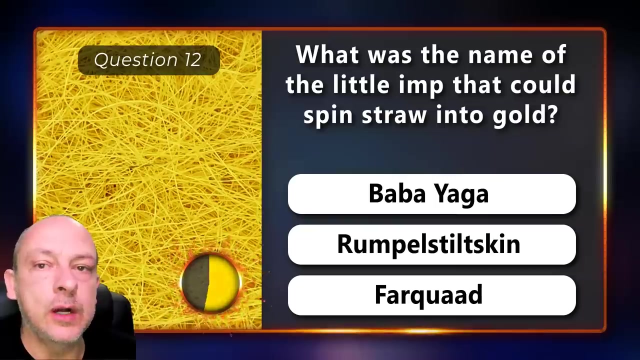 According to legend, which is the lost city of gold? El Dorado, Atlantis or Laurasia El Dorado? What was the name of the little imp that could spin straw into gold? Baba Yaga, Rumpelstiltskin or Farquad? 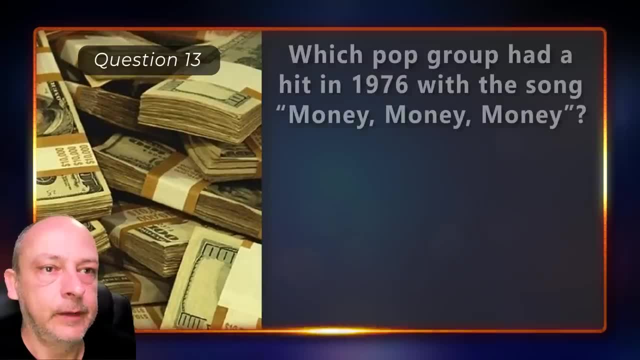 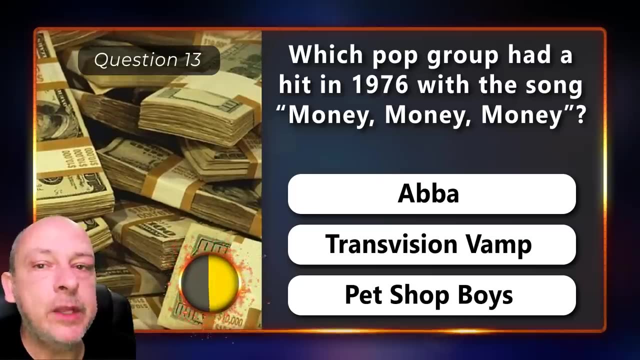 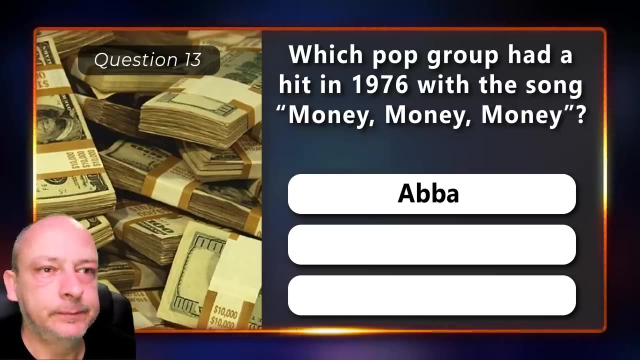 Rumpelstiltskin, Which pop group had a hit in 1976 with the song Money, Money, Money, ABBA Transvision, Vamp or Pet Shop Boys? And the answer is ABBA. Who was the first person ever to reach a personal? 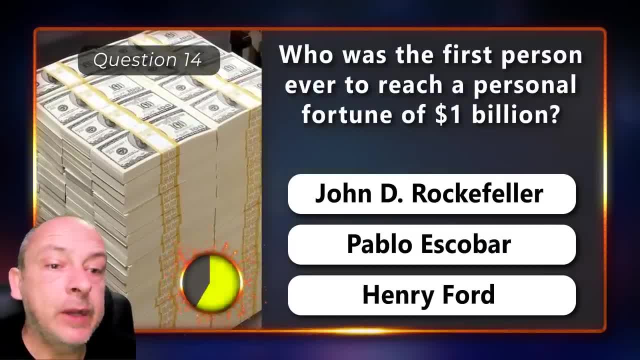 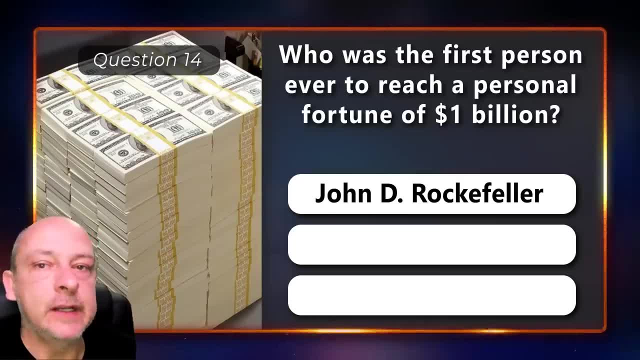 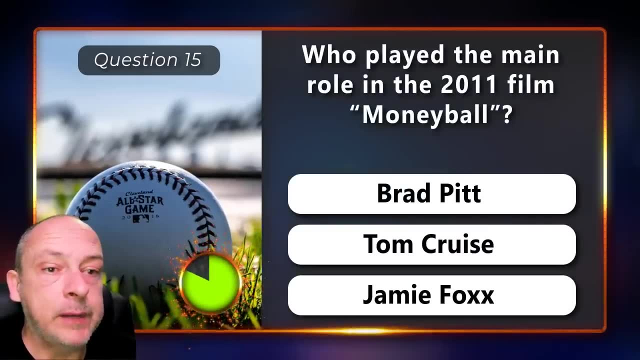 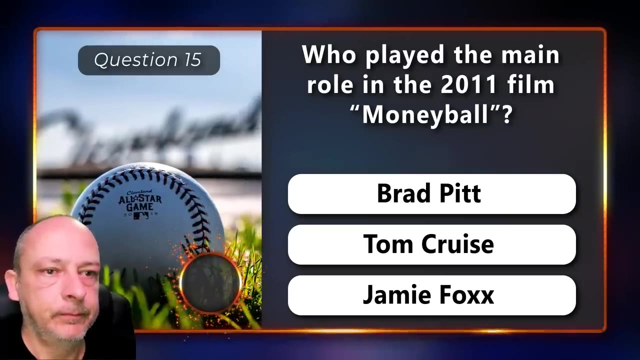 financial fortune of $1 billion. Rockefeller, Pablo Escobar or Henry Ford? John D Rockefeller, Who played the main role in the 2011 film Moneyball? Was it Brad Pitt, Tom Cruise or Jamie Foxx? The correct answer is Brad Pitt. 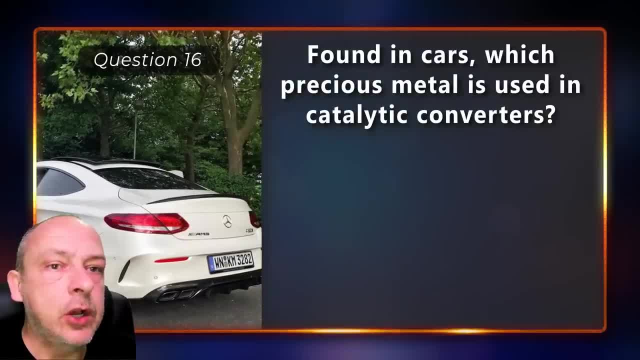 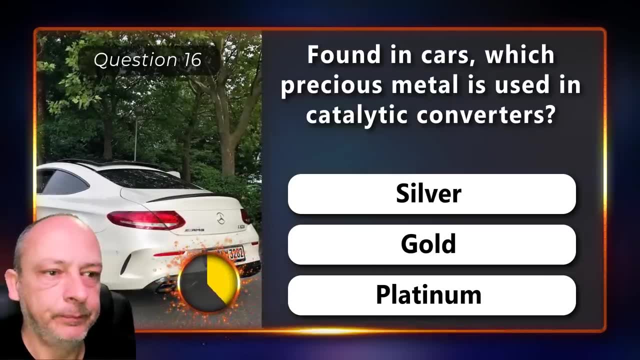 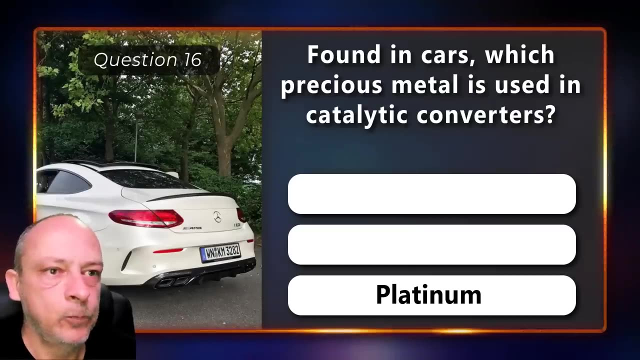 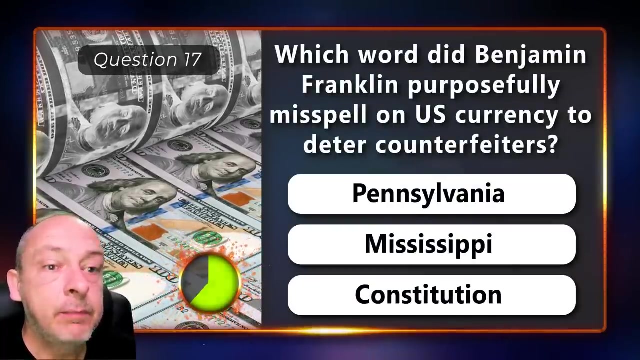 Who was the first person ever to reach a personal financial fortune of $1 billion Found in cars? which precious metal is used in catalytic converters? Is it silver, gold or platinum? Platinum is the answer. Which word did Benjamin Franklin purposely misspell on US currency to deter counterfeiters? Pennsylvania, Mississippi or Constitution? 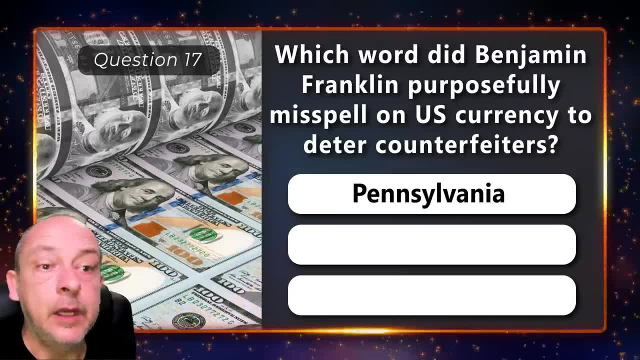 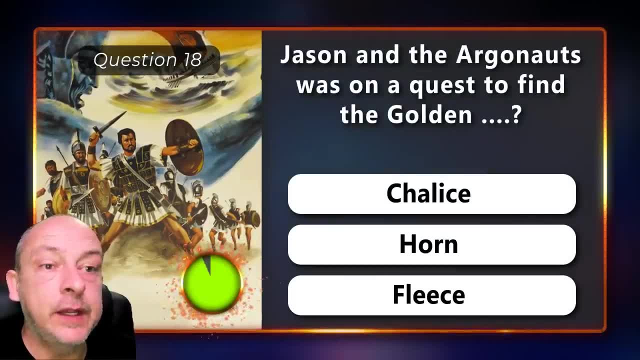 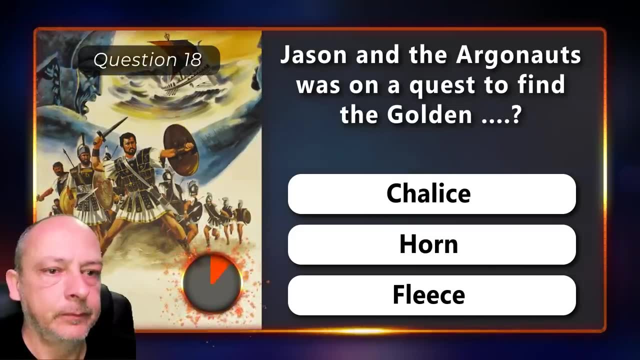 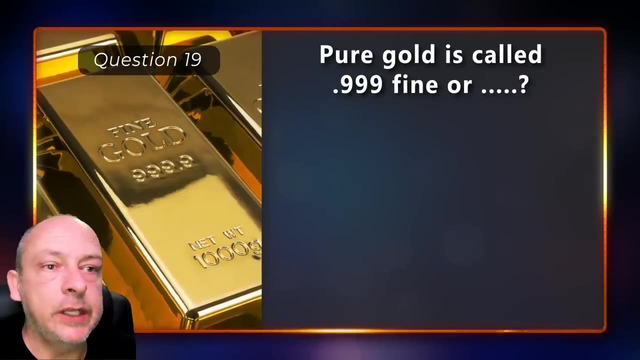 He misspelled Pennsylvania. Jason and the Argonauts was on a quest to find the golden chalice horn or fleece, The golden fleece. Pure gold is called .999 fine or 99 carat, 52 carat or 20 carat. 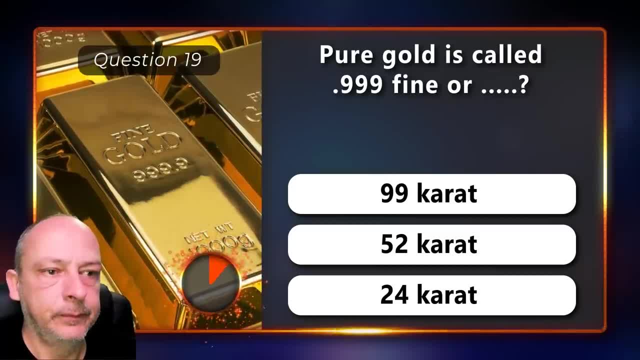 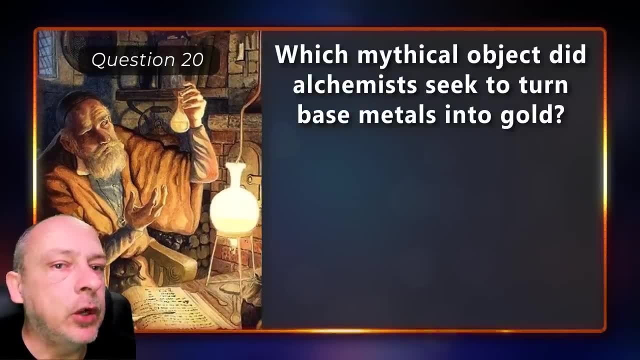 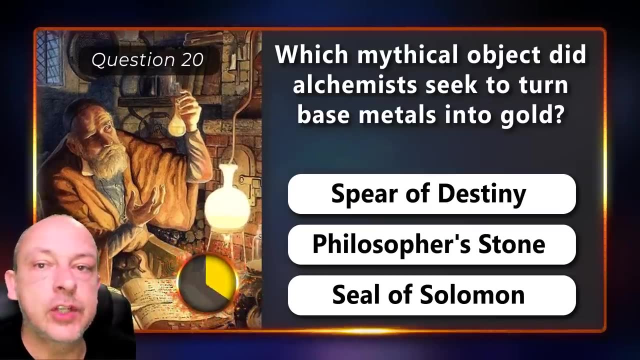 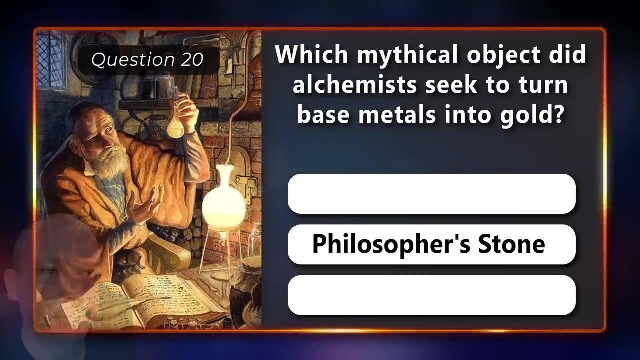 It is 24 carat. It is 24 carat. Which mythical object did alchemists seek to turn base metals into gold? spear of destiny, philosopher's stone or the seal of Solomon, The philosopher's stone? Did you know that pirates wore eye patches not because they had lost an eye in battle, but to help their eyes? 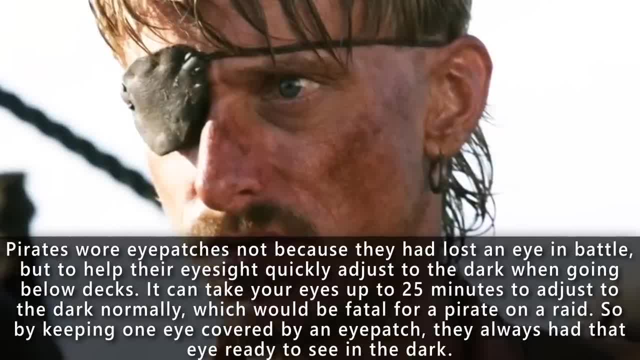 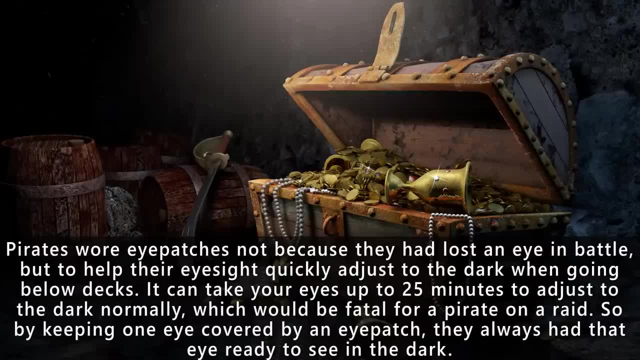 To help their eyesight quickly adjust to the dark. when going below deck It can take your eyes up to 25 minutes to adjust to the dark normally, which would be fatal for a pirate on a raid. So by keeping one eye covered by an eye patch, they always had that eye ready to see in the dark. 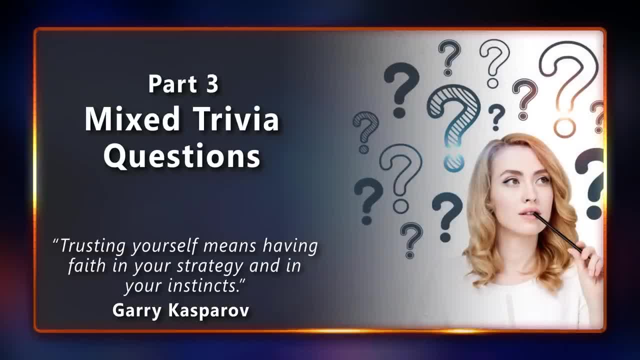 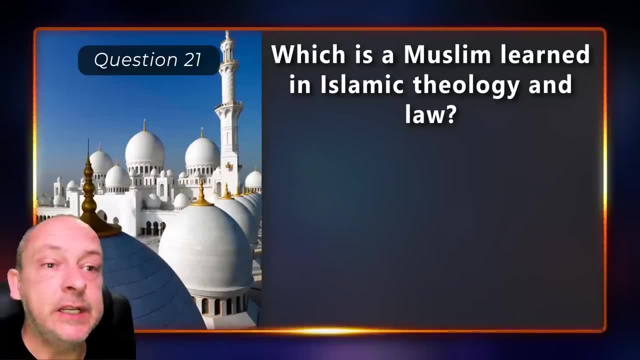 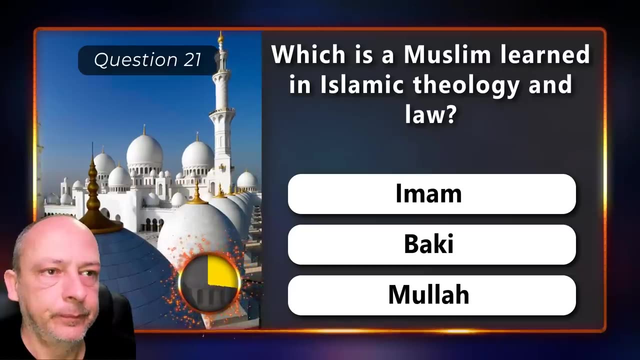 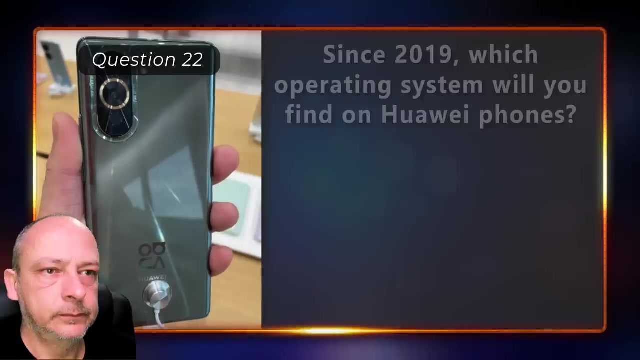 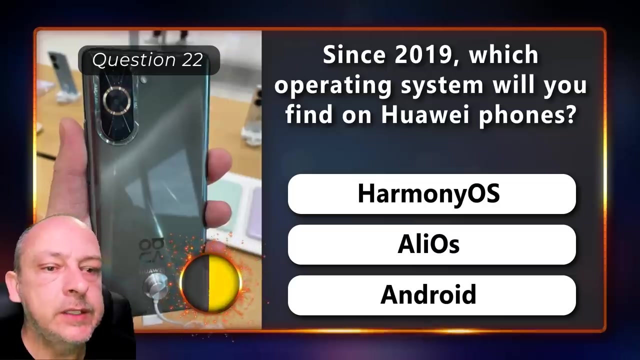 Which is a Muslim learned in Islamic theology and law- An Imam, a Baqi or a Mullah? Which is a Muslim learned in Islamic theology and law- An Imam, a Baqi or a Mullah? Subscribe for more. Since 2019,. which operating system will you find on Huawei phones? Harmony OS, AliOS or Android? 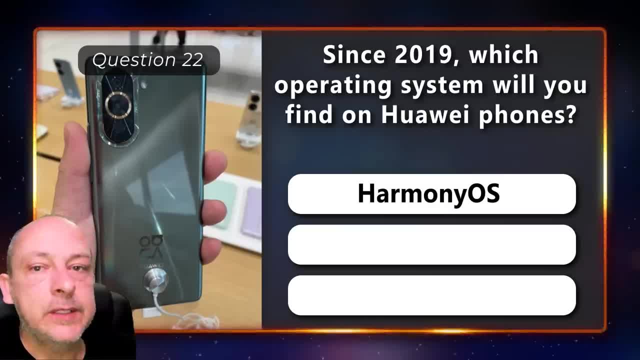 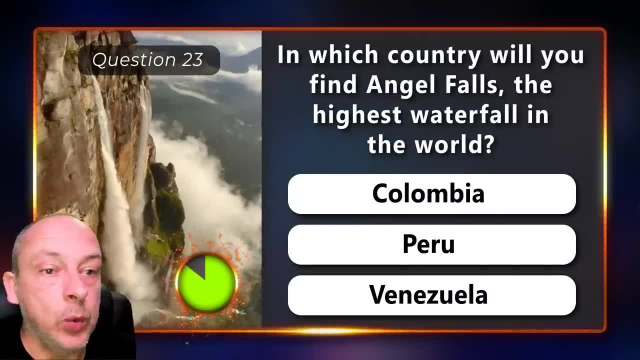 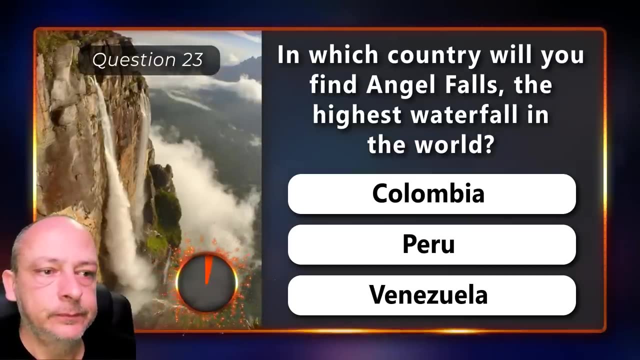 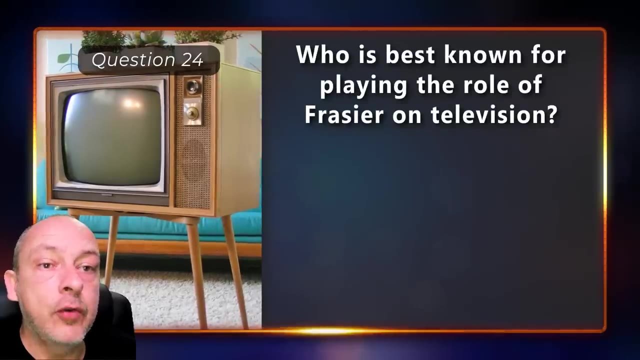 Harmony OS. In which country will you find Angel Falls, the highest waterfall in the world? Why Colombia, Peru or Venezuela? it is in Venezuela who is best known for playing the role of Frasier on television: Bryan Cranston, Ty Burrell or Kelsey Grammer. 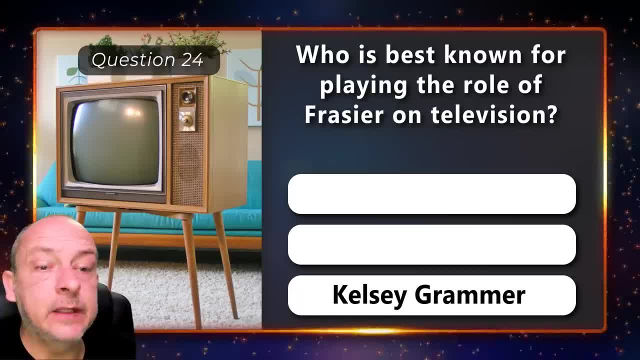 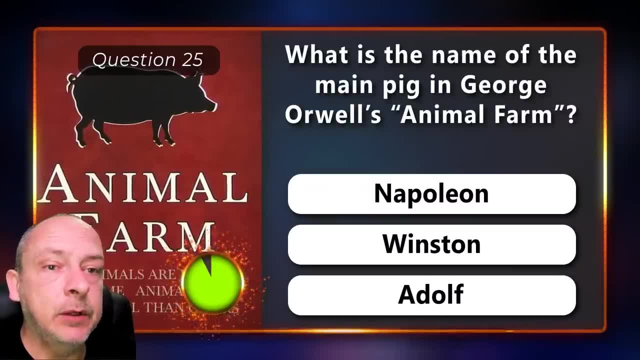 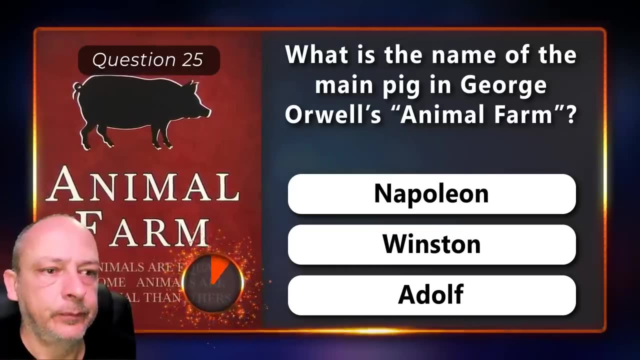 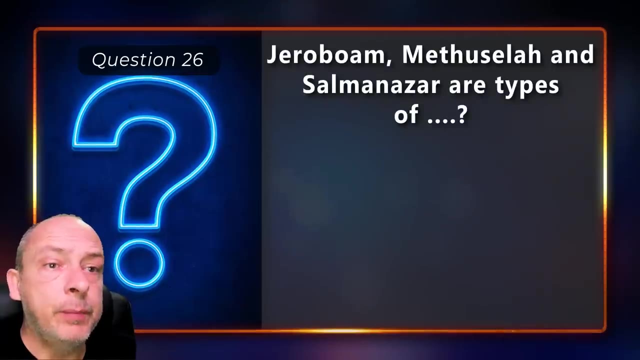 it is Kelsey Grammer. what is the name of the main peak in George Orwell's animal farm? is it Napoleon, Winston or Adolf? it is Napoleon. Jeroboam, matusole and Salman Azhar are types of knitting stitches. champagne bottles and other types of knitting stitches. 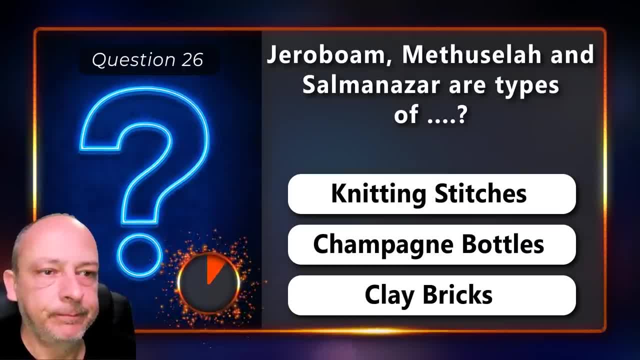 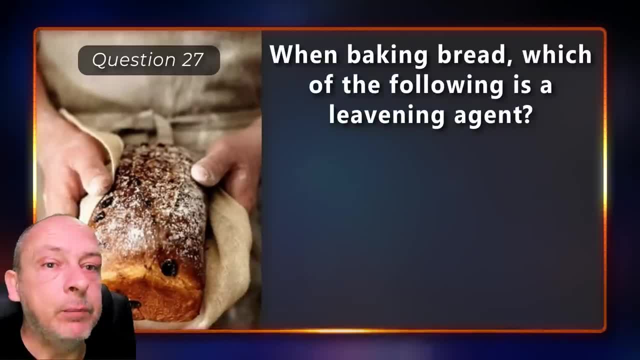 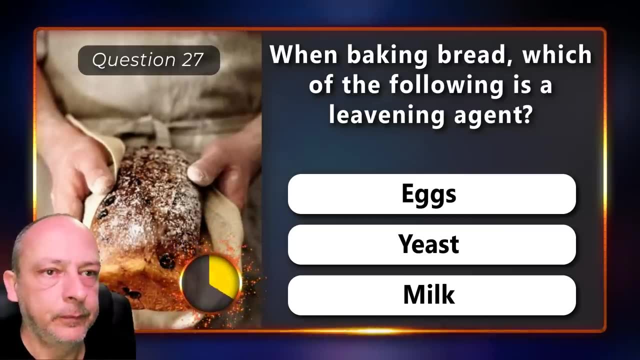 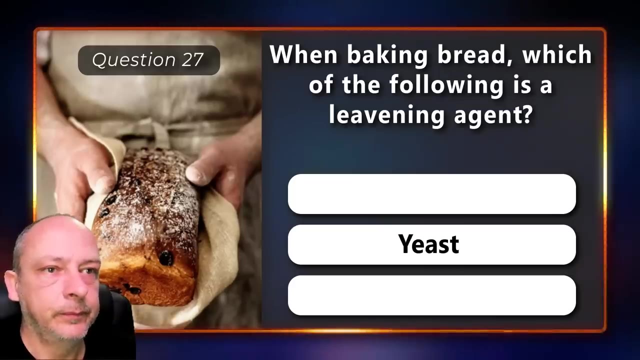 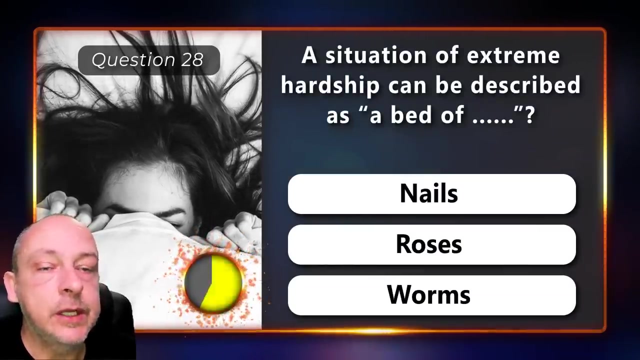 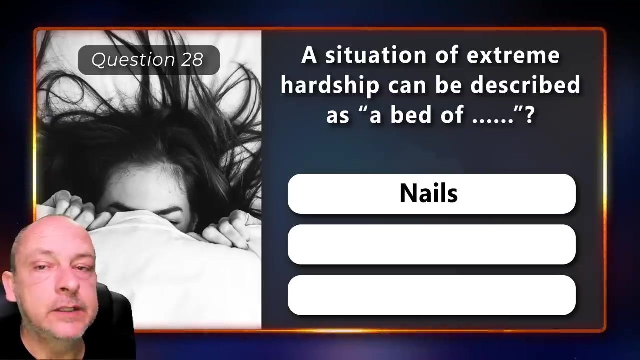 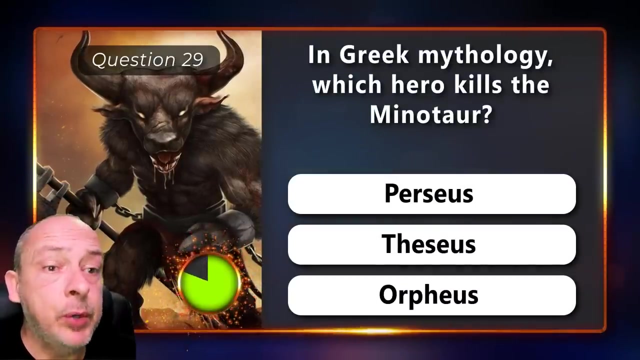 or clay bricks. it is champagne bottles. when baking bread, which of the following is a leafening agent? eggs, yeast or milk yeast? a situation of extreme hardship can be described as a bed of lice, nails, roses or worms. a bed of nails. in Greek mythology, which hero kills the minotaur? is it Perseus, Theseus or Orpheus? 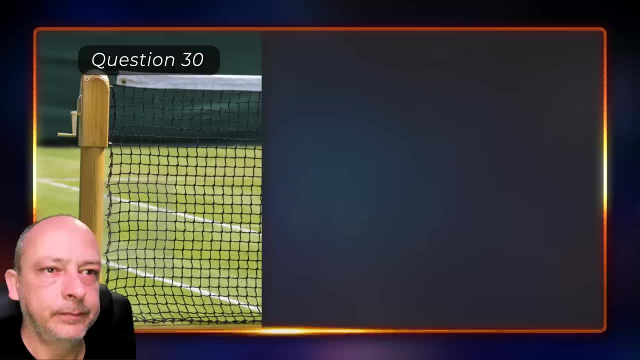 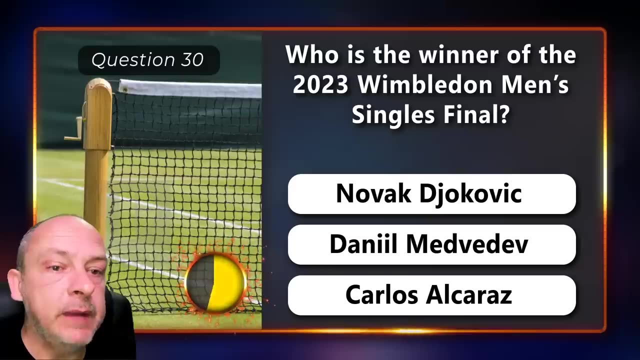 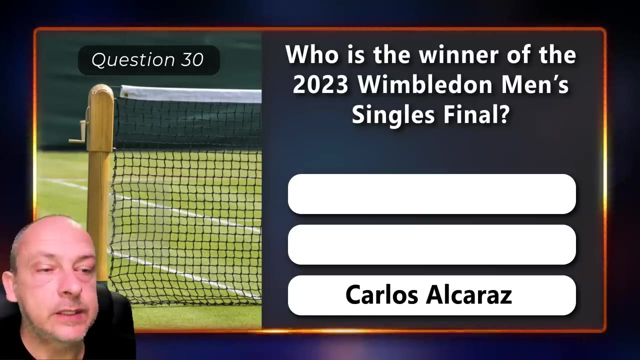 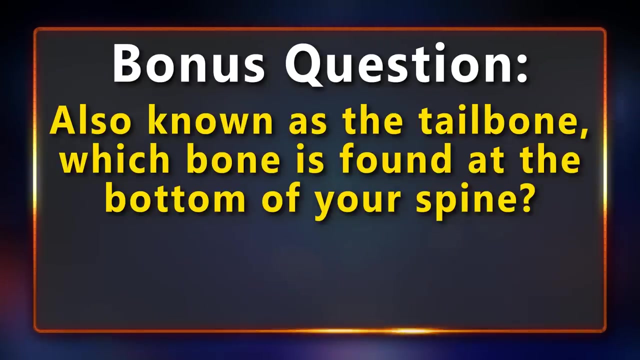 the answer is Theseus. who is the winner of the 2023 Wimbledon Men's Singles Final? is it Novak Djokovic, Daniel Medvedev or Carlos Alcaraz? Carlos Alcaraz? time for the bonus question, also known as the tailbone: which bone is found at the bottom of? 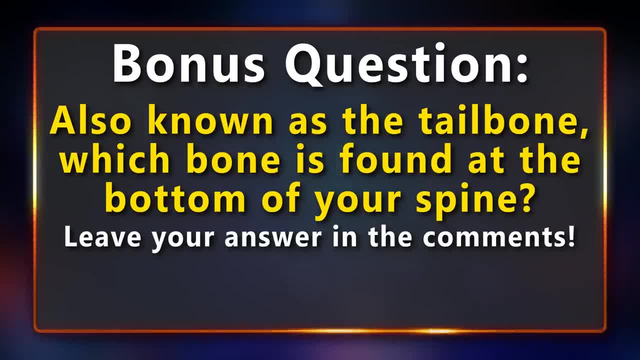 your spine. if you know the answer to this question, leave it in the comments. and if you are enjoying this quiz, please leave a like and consider subscribing. it really helps. now back to the quiz. we'll see you in the next video. see you in the next video. 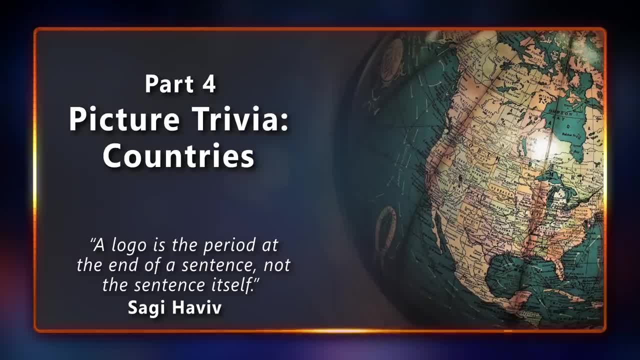 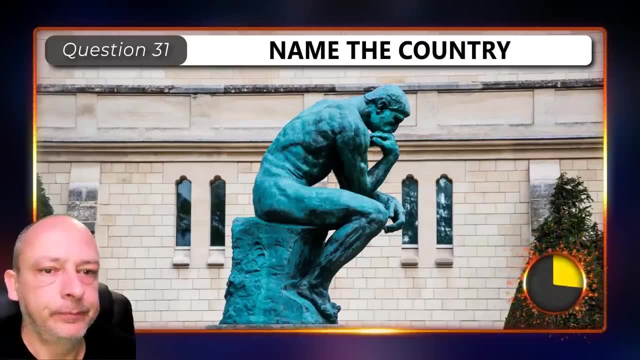 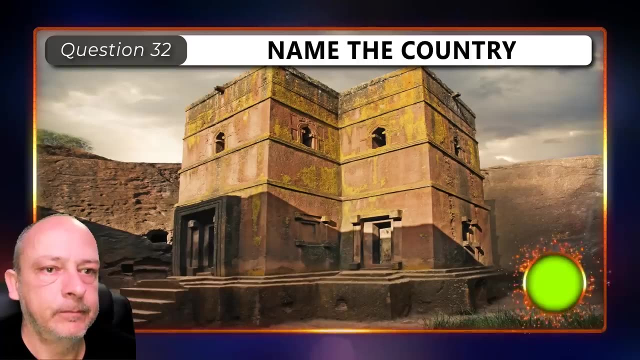 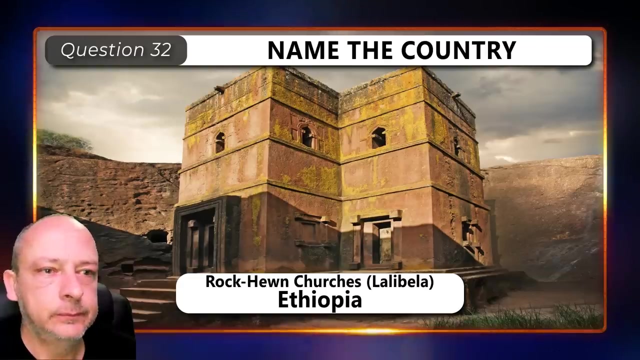 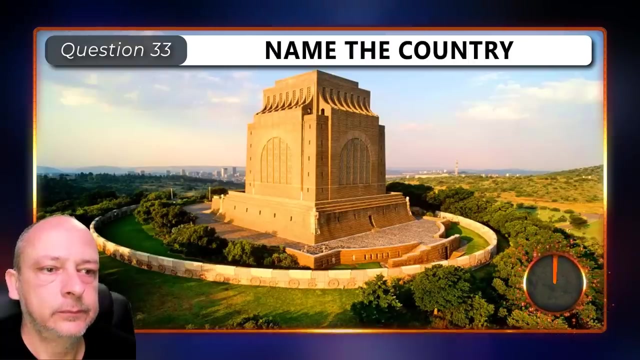 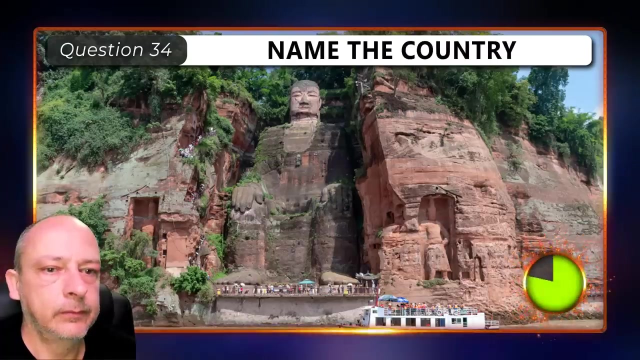 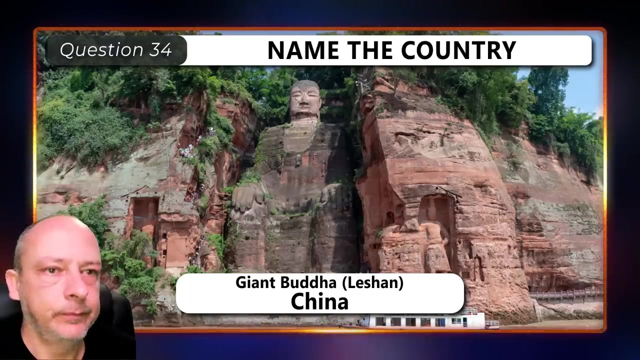 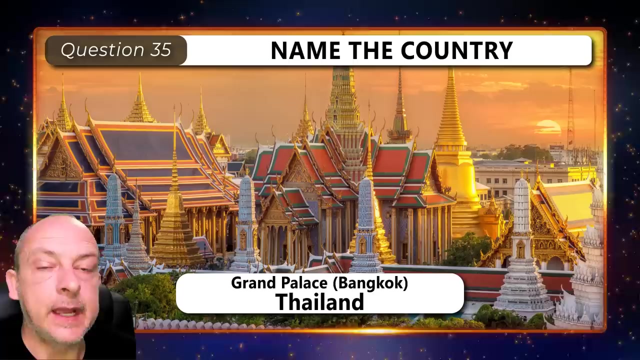 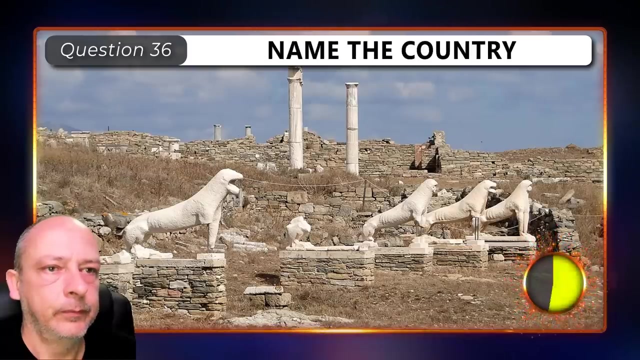 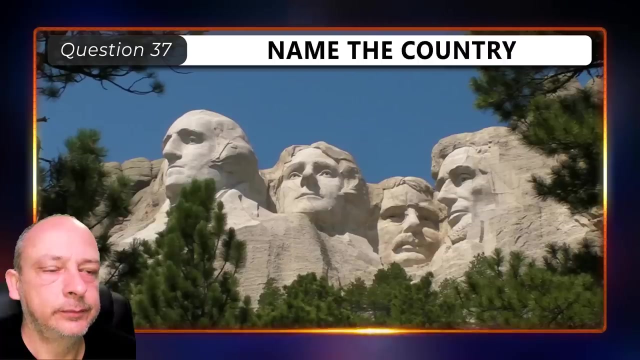 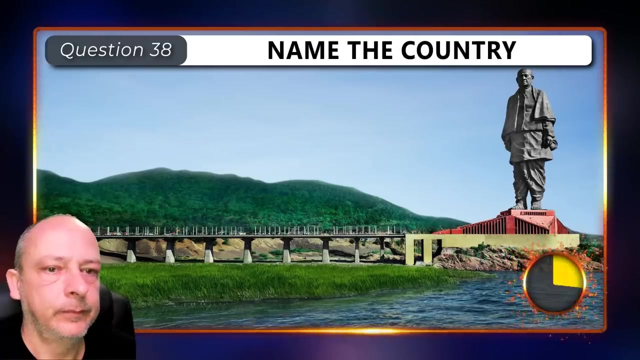 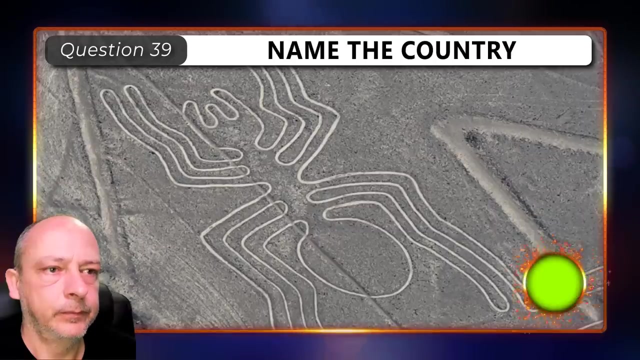 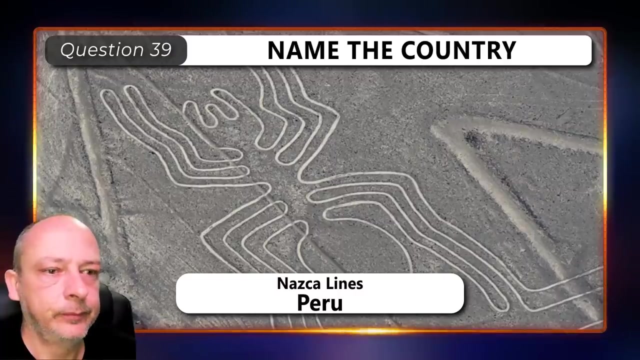 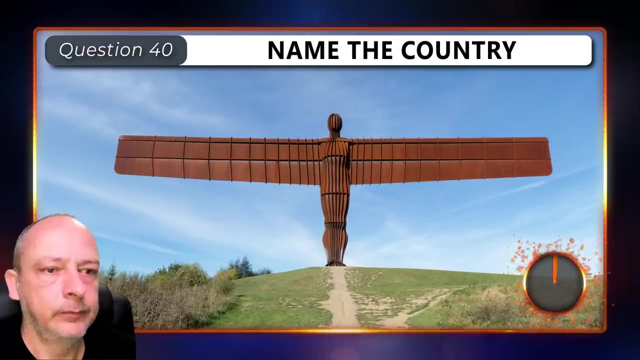 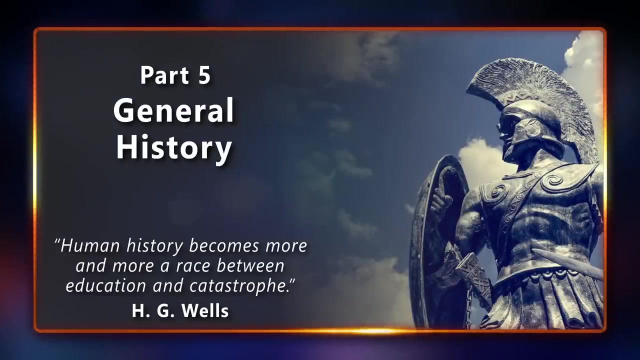 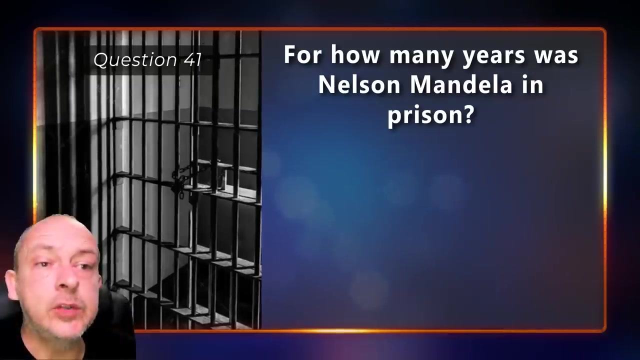 see you in the next video. identify each country from the landmark: France, Ethiopia, South Africa, South Africa, China, Thailand, Thailand, Greece, Greece, USA, India, India, Thailand, India, Mexico, Peru, Peru, Mexico, Mexico, Mexico and England and England and England. England and England, England, Africa and the United States, Argentina, Brazil. 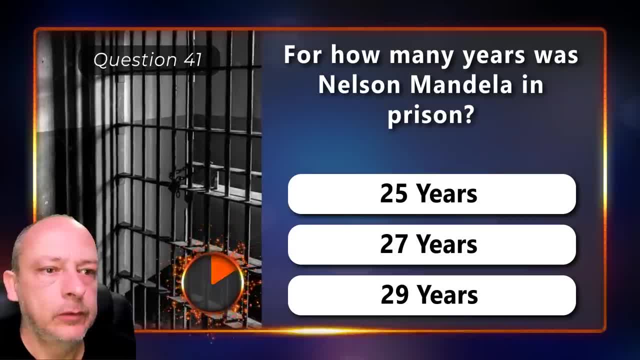 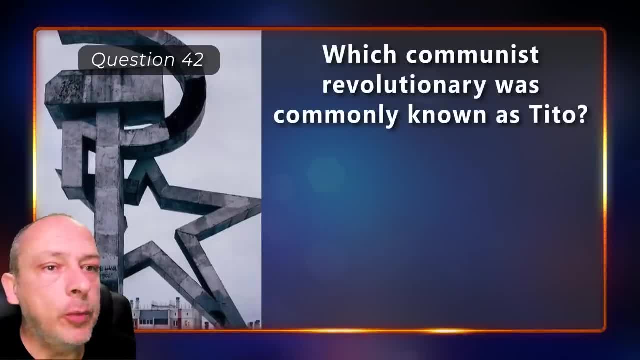 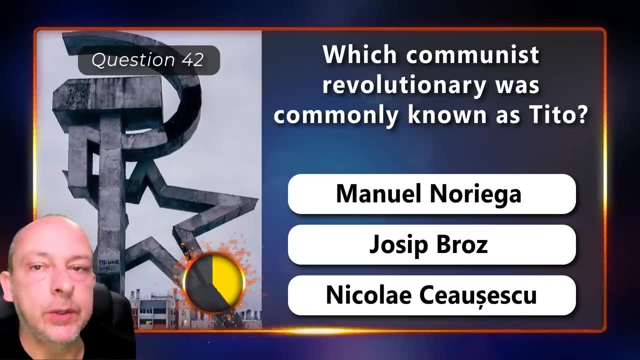 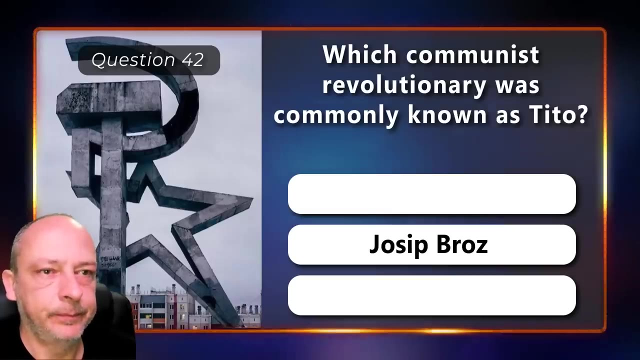 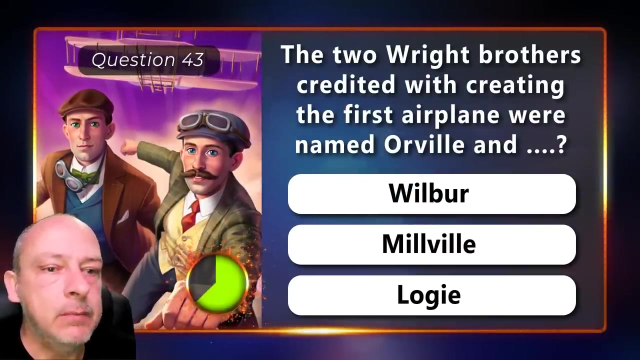 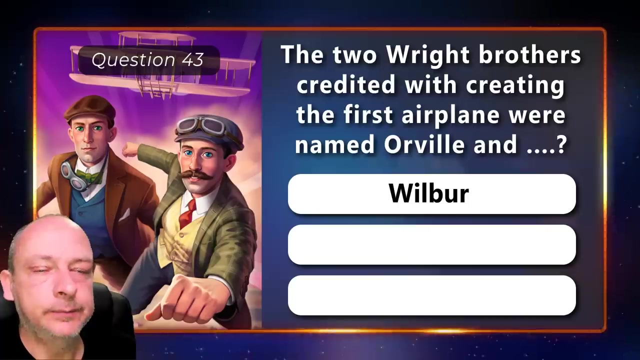 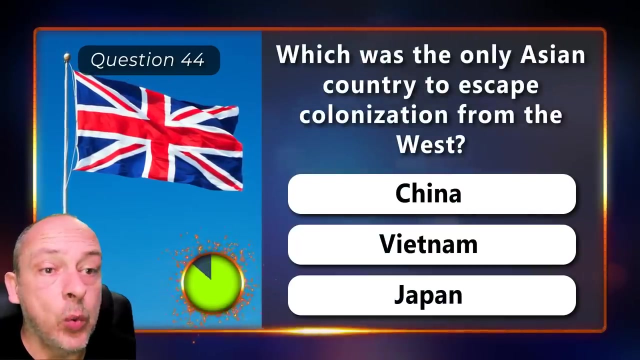 Brazil, Europe, Japan, South Africa, Brazil, California, China, Mexico, Australia, uish Brazil. The two Wright brothers credited for creating the first airplane were named Orwell and Wilbur Millville, or Logie Wilbur, Which was the only Asian country to escape colonization from the West China Vietnam.